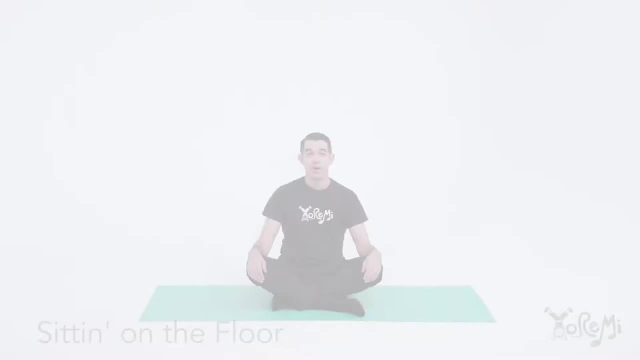 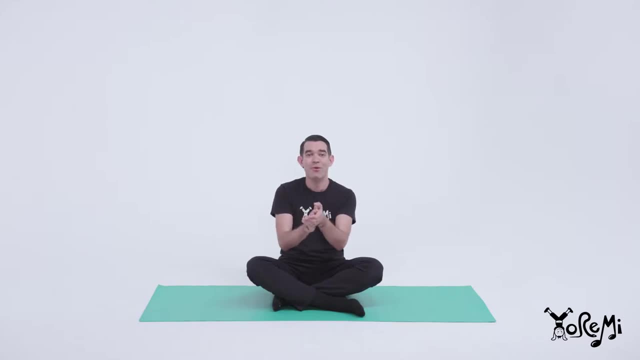 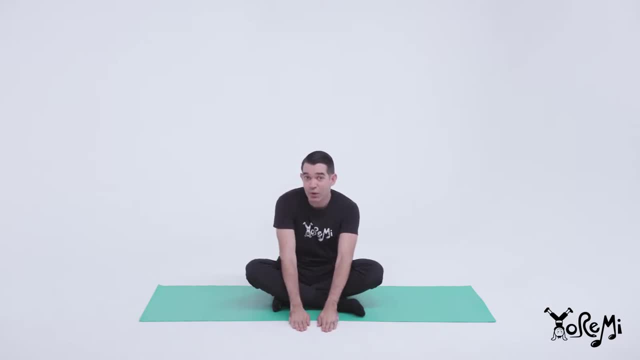 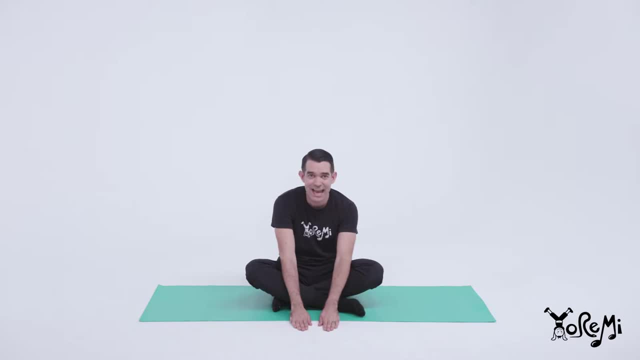 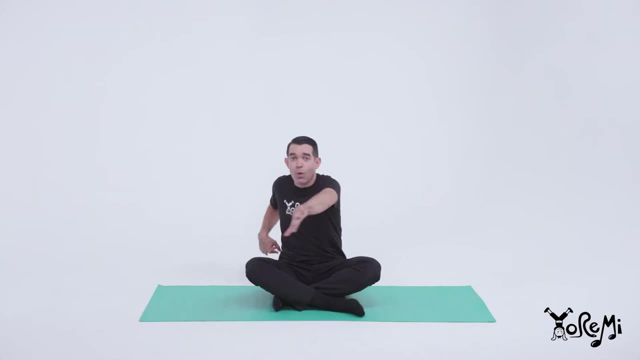 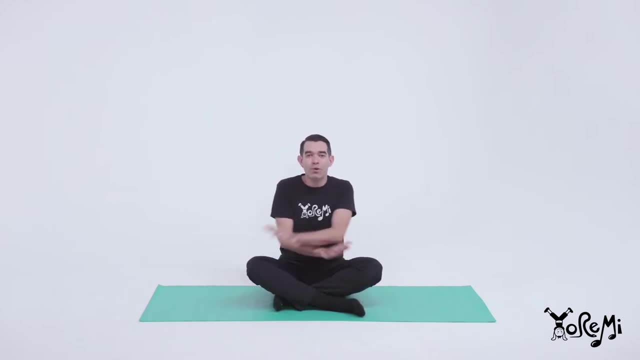 You can't do nothing sitting on the floor. No, you can't do nothing sitting on the floor, But I can- oo-ah, oo-ah sitting on the floor. I can oo-ah, oo-ah sitting on the floor.